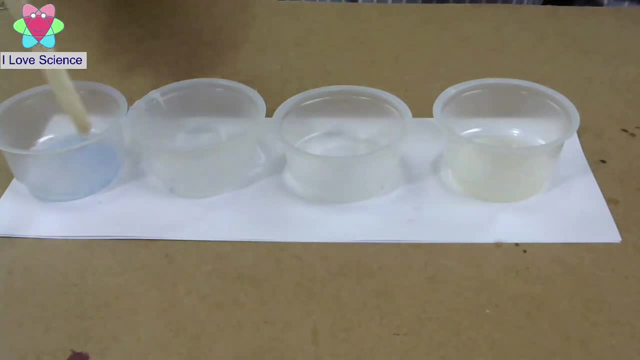 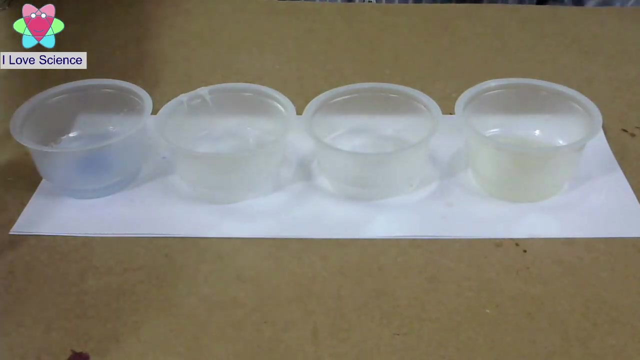 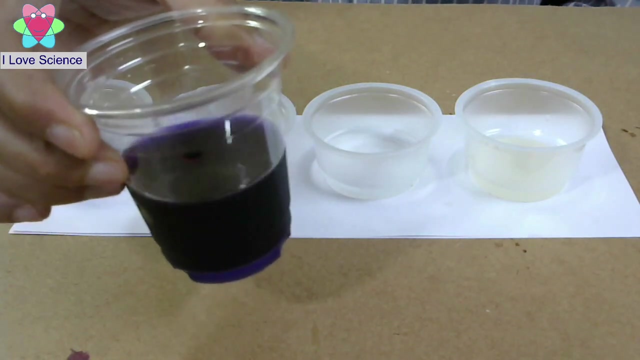 this And then we will mix them. Let's see. Okay, Okay, Okay. So let's use different stirrer for acids and bases. So our four samples of acids and bases are ready Now. this is our natural indicator. Now do you know what is this indicator? You must have seen purple color cabbage like. 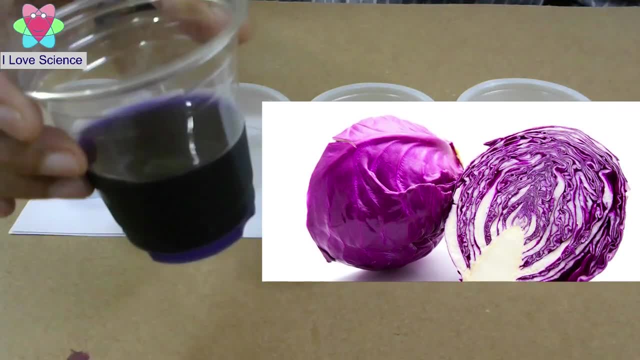 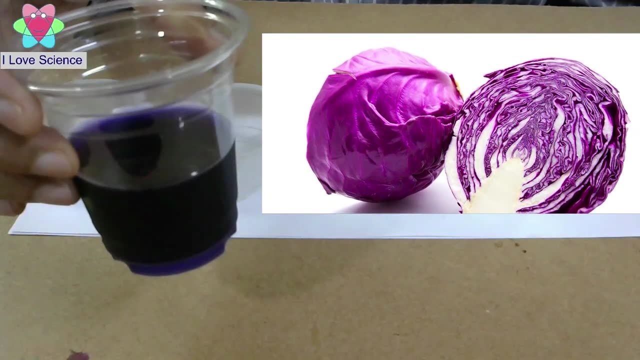 what you see on screen right now. Okay, Now, if that purple color cabbage you can buy from a vegetable shop, And then a few leaves of the purple cabbage you can put them in hot water, then, you know, extract the juice from that, then it becomes the purple juice. 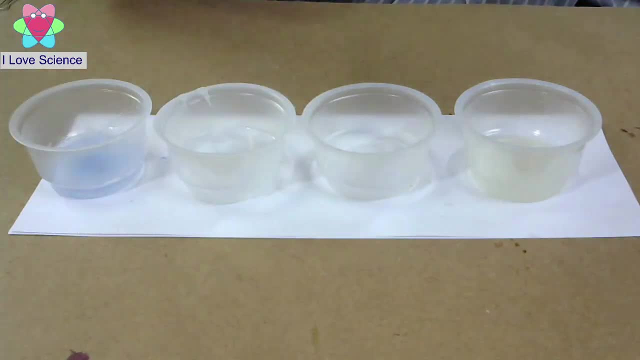 like this. now let's see how good is this? a purple indicator. so let's put that in some acid. lemon juice in the citric acid. okay, now you see both of them turn pink or red because acid changes the color to red. now let's put the same purple. 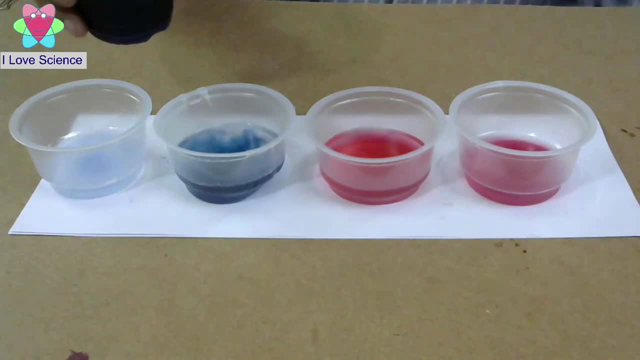 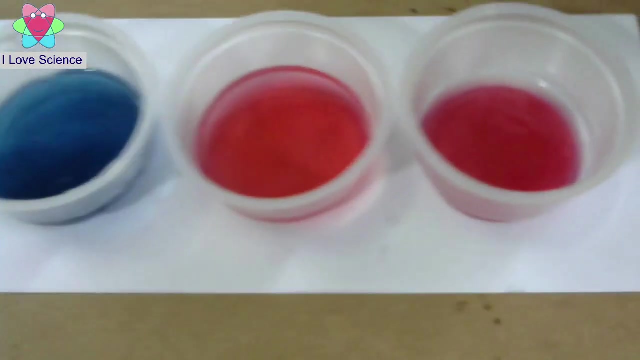 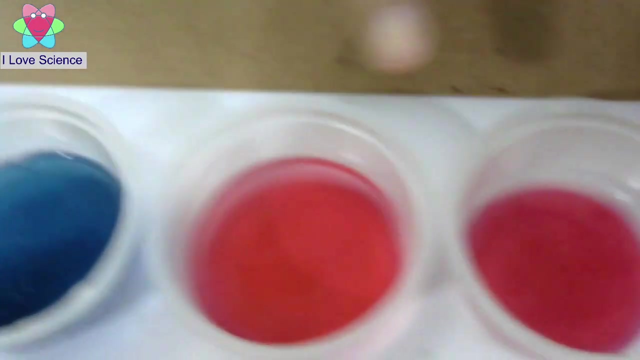 cabbage juice in baking soda and you will see that this becomes blue. it means it's a strong base. and in the detergent solution, now this becomes green, so this is also base. so now you can see this, that the color of these four indicators- lemon juice, citric acid, baking soda and detergent. so you can see very clearly. 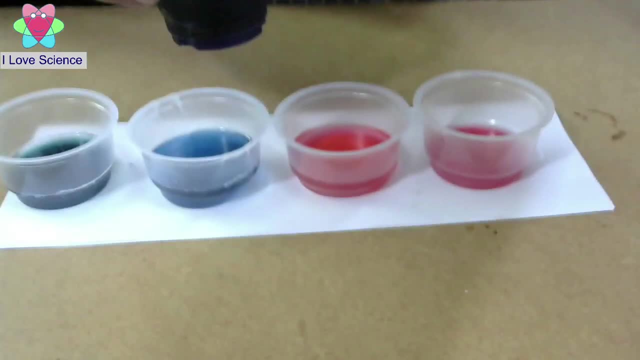 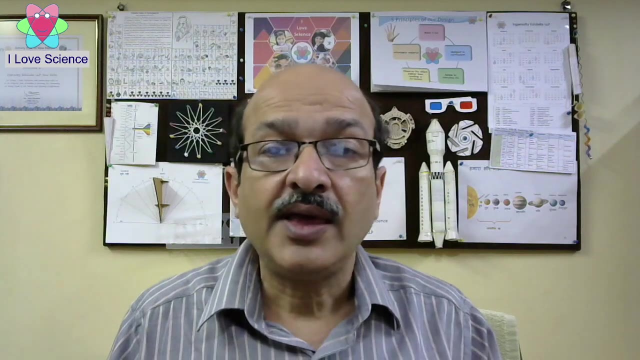 that our same indicator that we have okay, has a blue base and a green base. so now you can see that the color of these four indicators change the color of these different solutions as per their acid or base nature. another natural indicator which can change color to identify bases is: 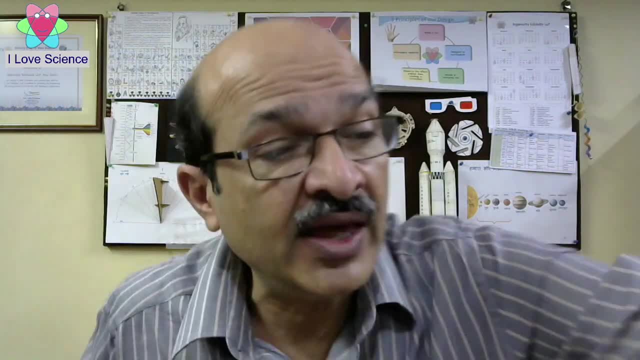 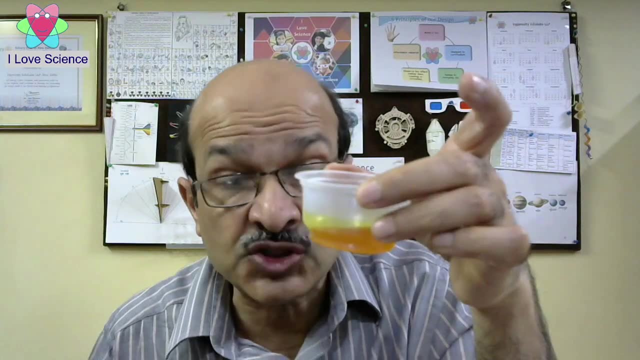 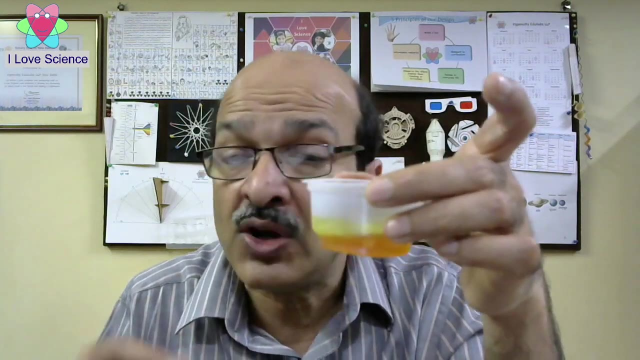 haldi or turmeric. okay, so what we have done? so here we have taken some turmeric powder. you can take it from your kitchen and then dissolve it in the alcohol or maybe the hand sanitizer- right, because haldi does not are very good for our skin. so, for example, if you take this turmeric powder, 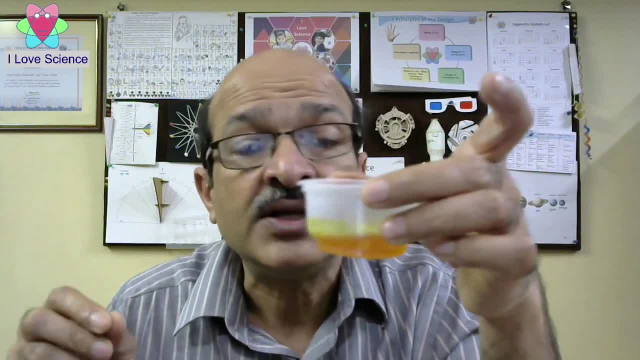 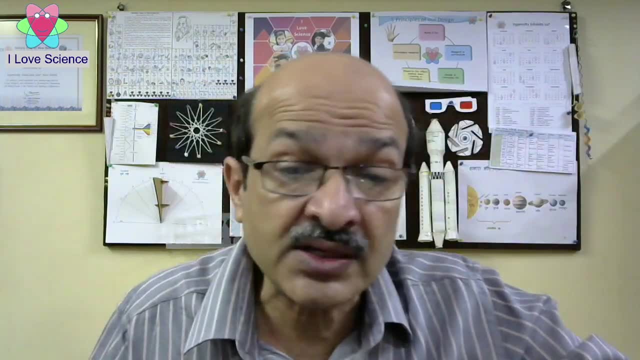 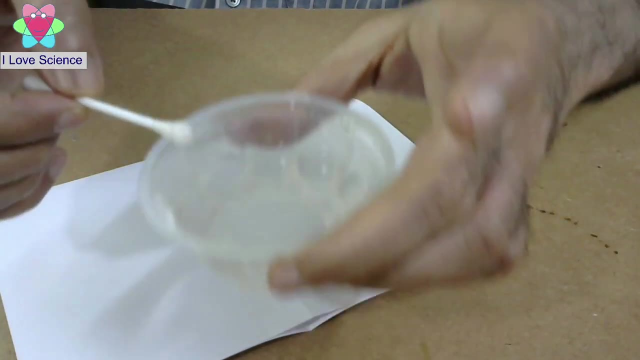 dissolve properly into pure water. it's difficult, so it is better to dissolve it in the hand sanitizer, because it has some alcohol and then it becomes a yellow solution like this. now let's see how can we use it to test base indicators. so in this small cup we have dissolved some baking soda into water. so 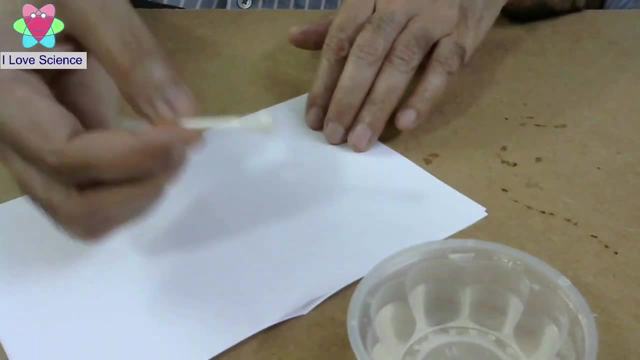 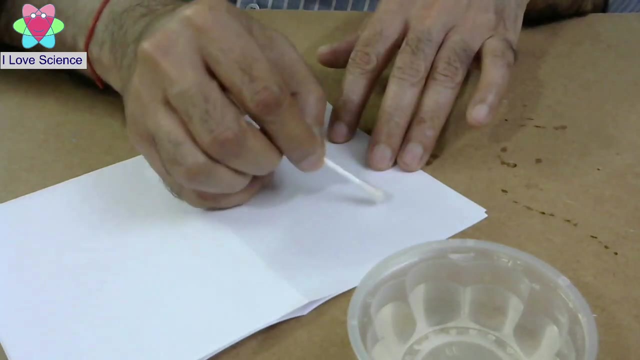 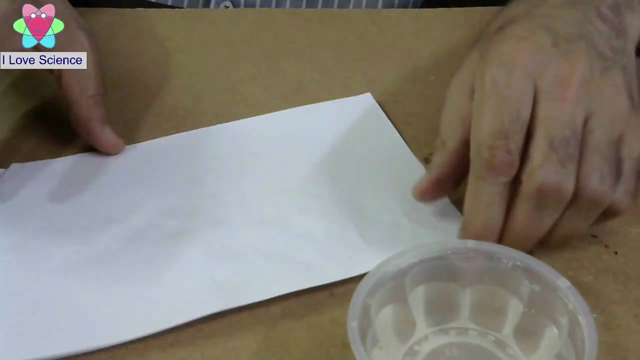 that this solution is basic. you, using a cotton swab, we can write something on this and it will be invisible, because this is this solution has no color, so I can write something which will not be visible. okay, so, and then let the paper dry. so here, on this paper, we have already written something using the 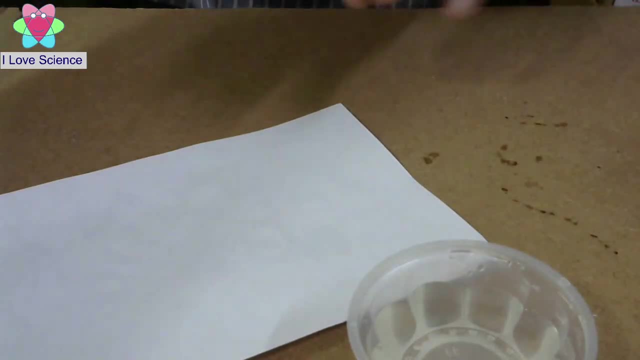 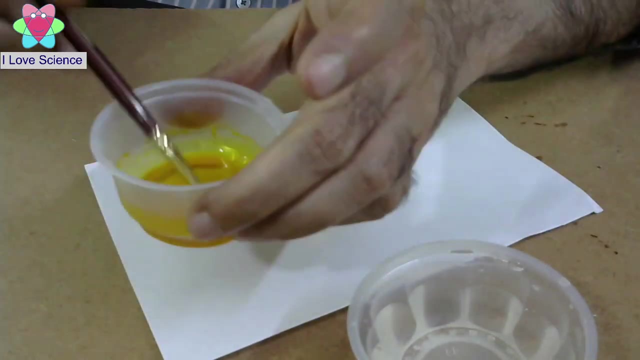 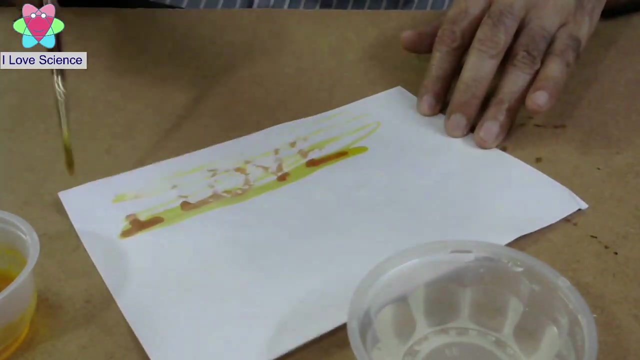 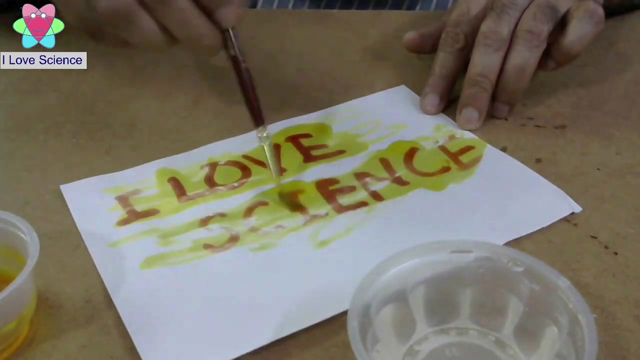 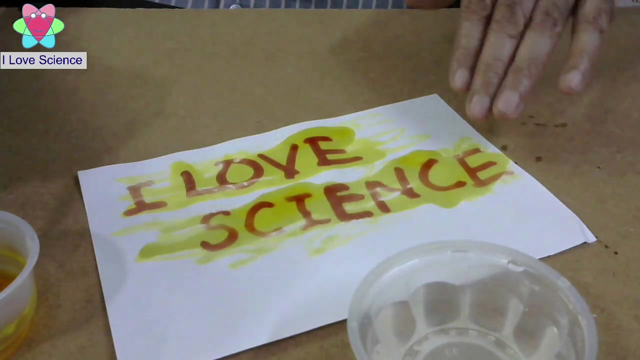 baking soda solution and now the paper is dry. now, if we want to see what is written on this, what we can do, we can take the turmeric solution and, using a brush, we can just write on this and then see if the color comes out. so can you see that the whatever was written on the paper with baking soda? 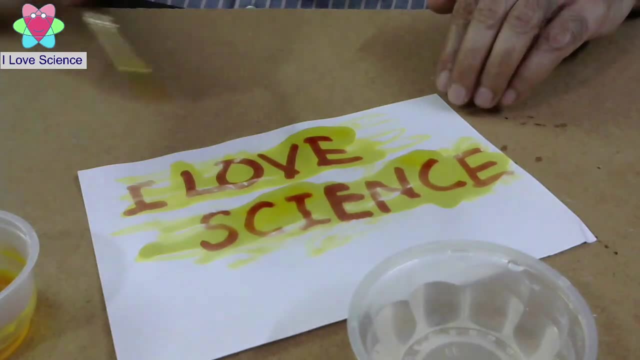 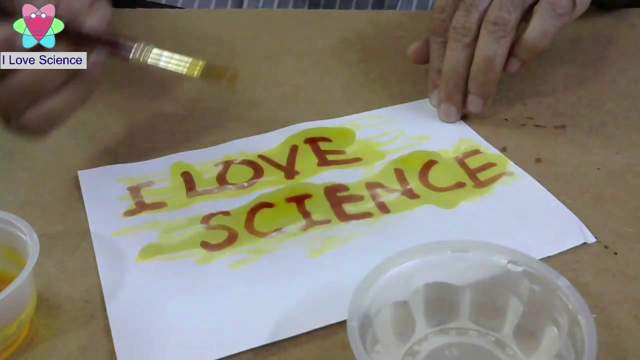 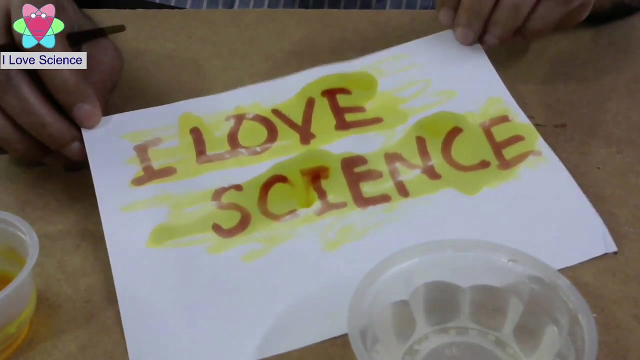 that much paper has turned red because the turmeric indicator turns into red when it comes in contact with base and because baking soda is a basic solution, then it becomes red. so this is how you can do your own experiment of this solution. so in this particular experiment we have used some of the 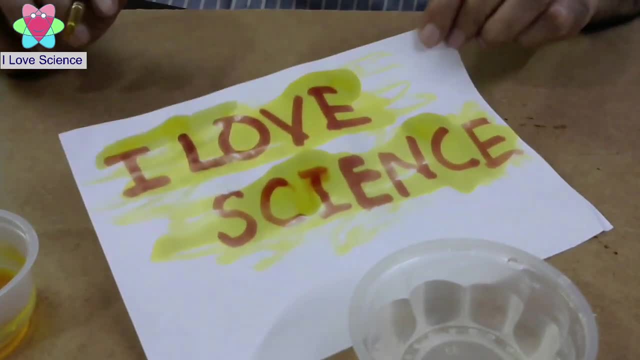 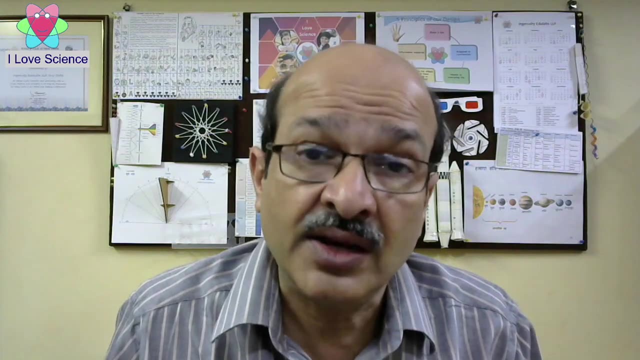 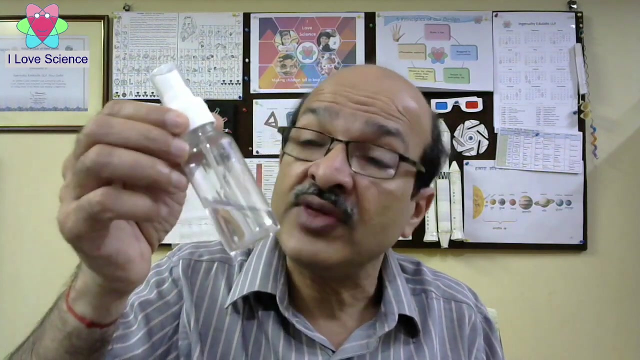 turmeric solution to identify, which is written on the paper. now in the next experiment we will use another indicator which changes color when it comes in contact with a base. now that indicator is phenolphthalein. so in this bottle we have taken some phenolphthalein and then we have put it in the spray bottle. now 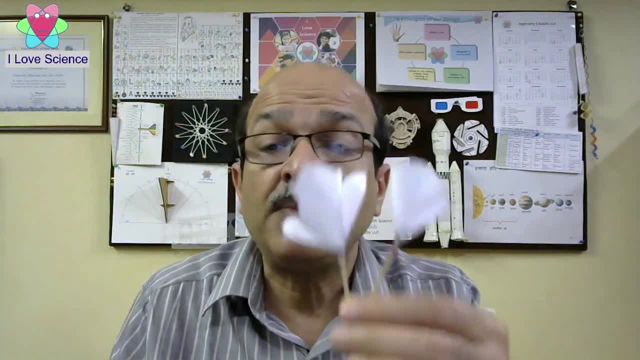 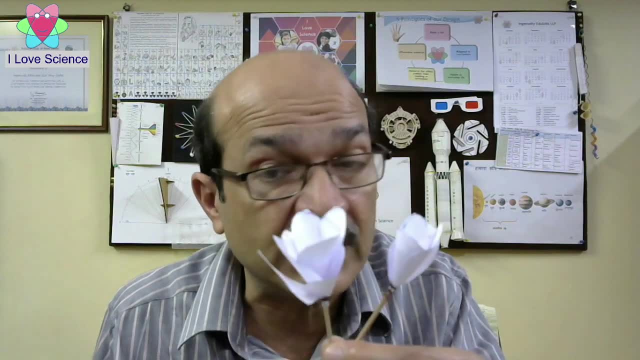 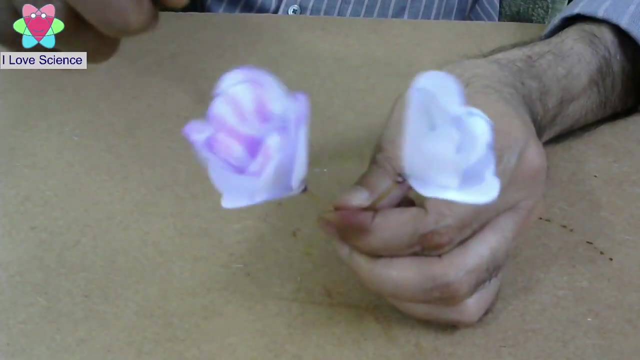 to test this. what we have done here. we have made some paper flowers from white paper and then put some baking soda solution on these. now let's see if we spray the phenolphthalein solution on these flowers, then what happens. and let's see if we. 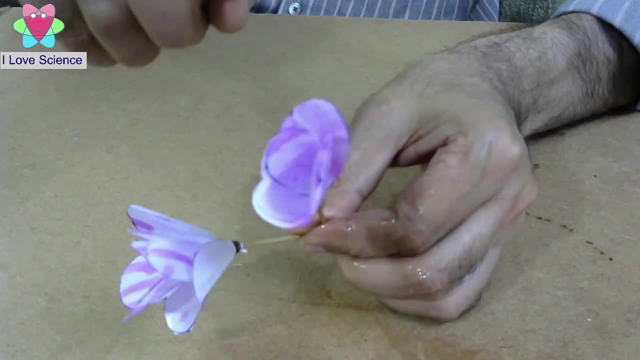 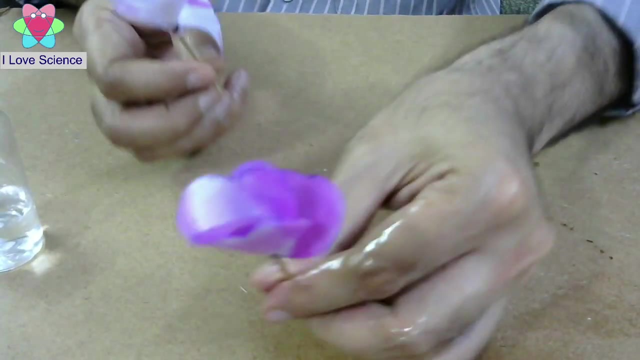 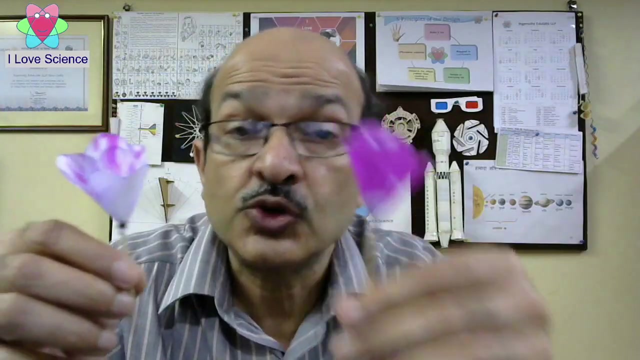 can change the color of these flowers and you can see that the solution becomes pink. and, as you can see here, these flowers become pink when they come in contact with phenolphthalein solution. so you can see these beautiful flowers and then how they turned from white to purplish pink. 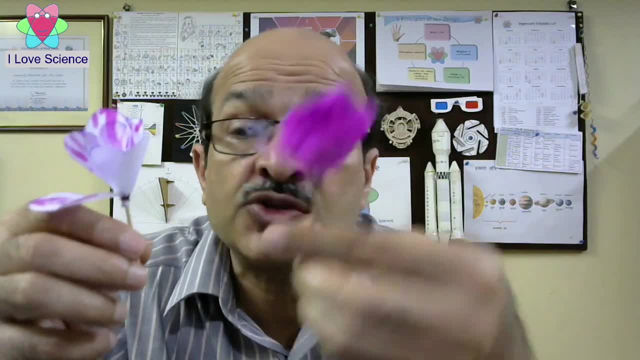 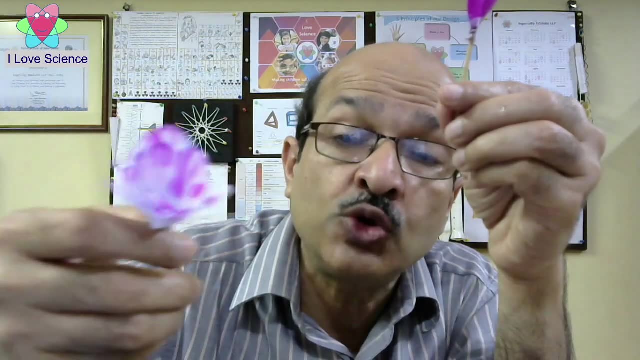 because this one we had dipped in the baking soda solution and on this one we had put some strokes of baking soda using a brush, so it only those parts have become pink, and this one has become pink all over. so this is how, using the phenolphthalein solution. 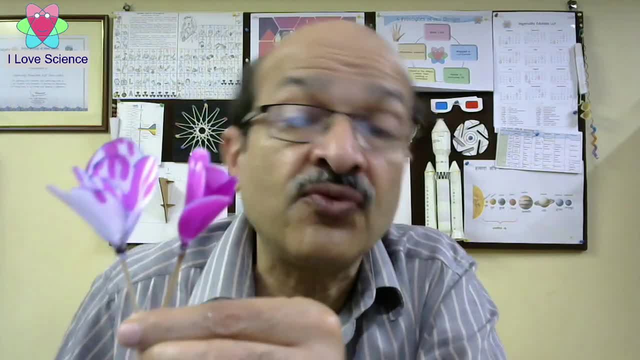 you can change the color of these flowers and then you can see how they turn from white to purplish pink. you can do some magic and then change the color of white flowers. you can also take natural flowers and then do the same experiment with them if the natural flower is white. 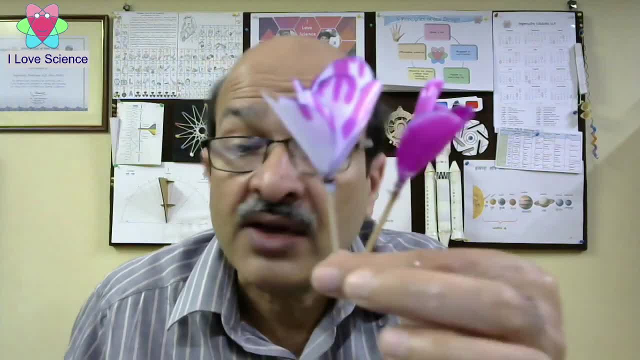 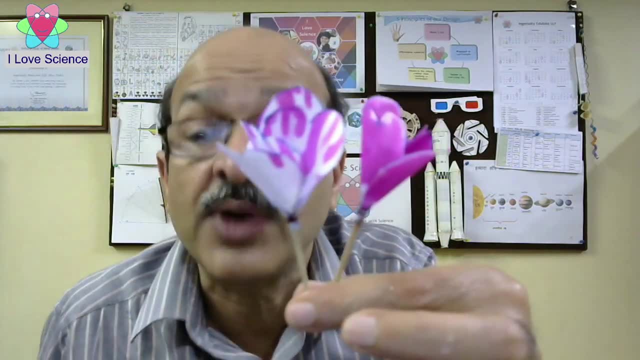 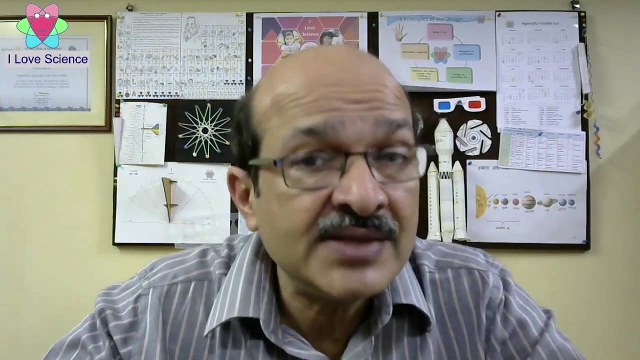 you can spray some baking soda solution when it becomes dry. after that spray the phenolphthalein solution and then you will see that the flowers become pink or purplish pink. in our next experiment we will do a simple reaction of acid and base and then see from that reaction the, if, the 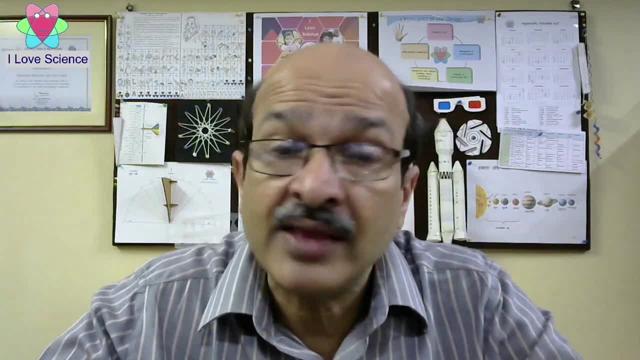 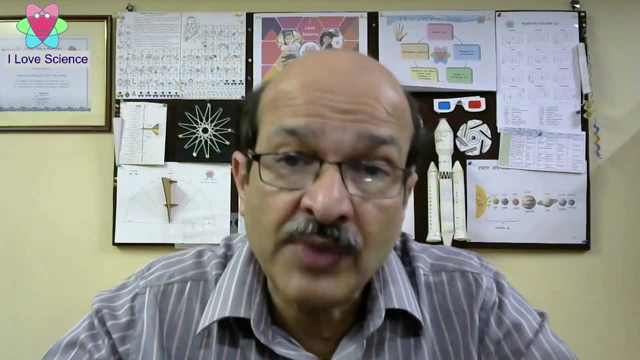 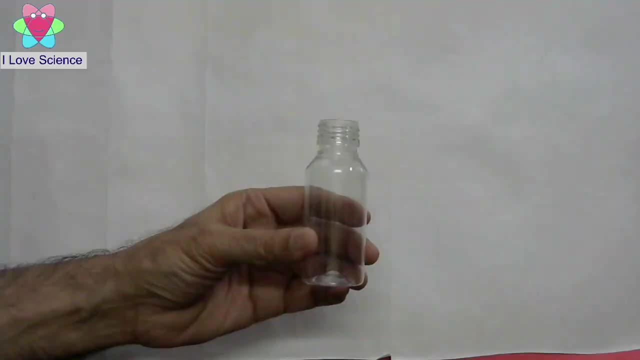 gas comes out, then how does the reaction happen? and this reaction you can do at home, because we will be using baking soda and citric acid. you will definitely have baking soda at home in your kitchen and if you do not have citric acid, you can also use lemon juice for this experiment. so for 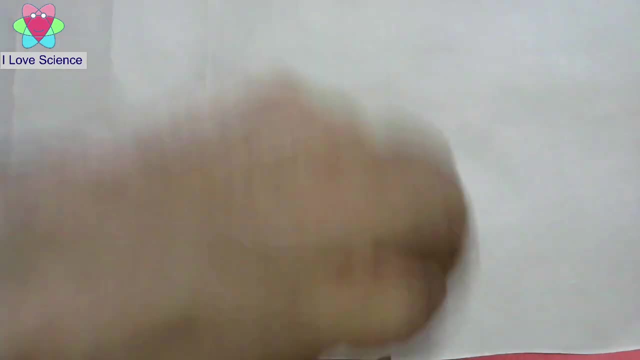 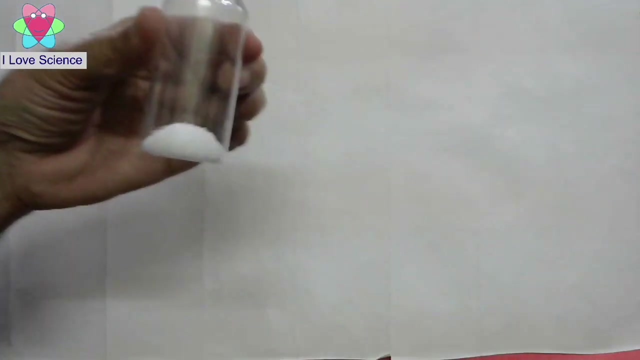 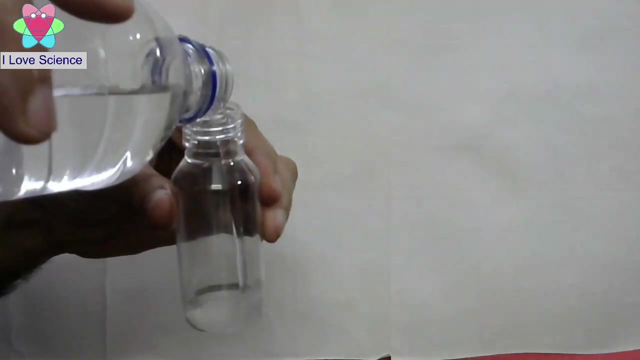 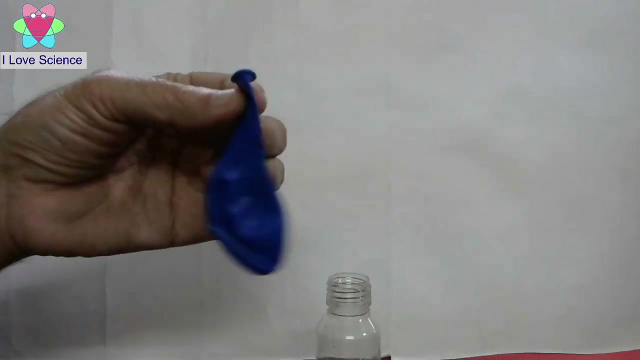 this experiment. we are taking some citric acid and, as i said, if you do not have citric acid, you can use some lemon juice for this purpose. so we have taken this much citric acid here. we will put some water in this to make a solution and let it mix. now we will fill the baking soda. 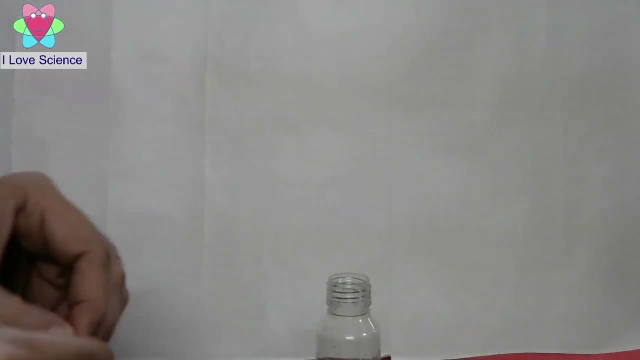 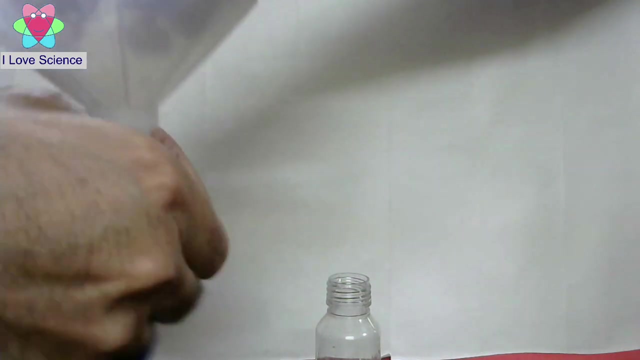 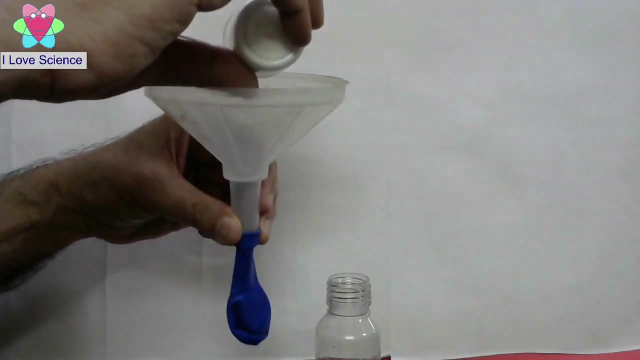 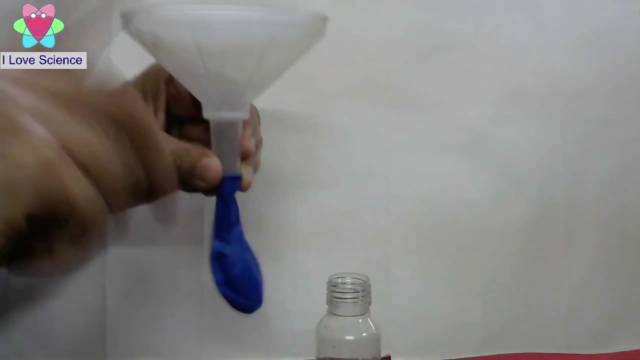 in this balloon, and you will see why i am doing that. so for filling the baking soda, we are just putting a funnel on the mouth of this balloon and then about one spoon of baking soda we will put in this. so all the baking soda has gone inside the balloon now. 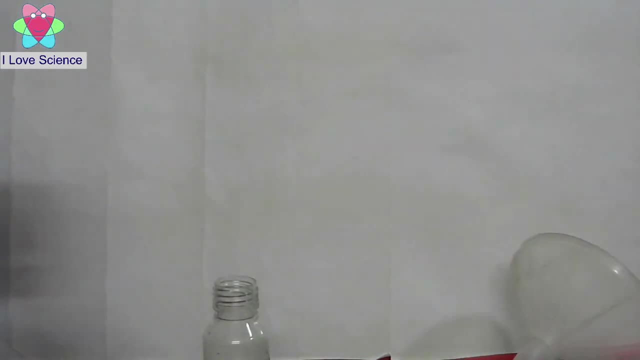 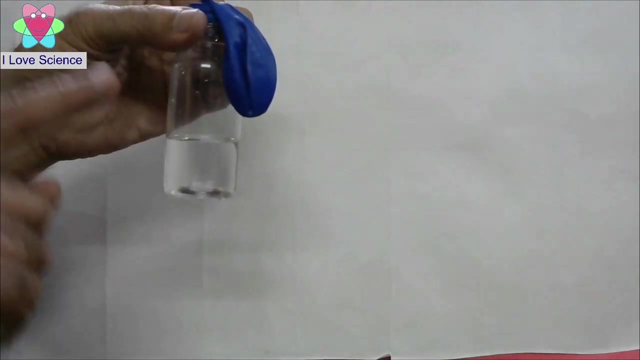 now we will fix the balloon on the mouth of the bottle so that the baking soda does not go inside a bottle till we close the mouth. now, this is ready now. if we let the baking soda go inside the citric acid, then let us see what happens. 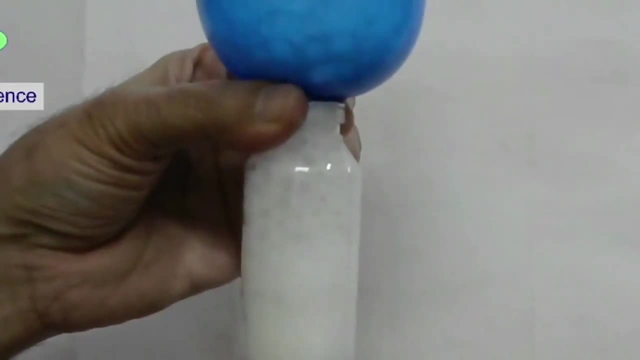 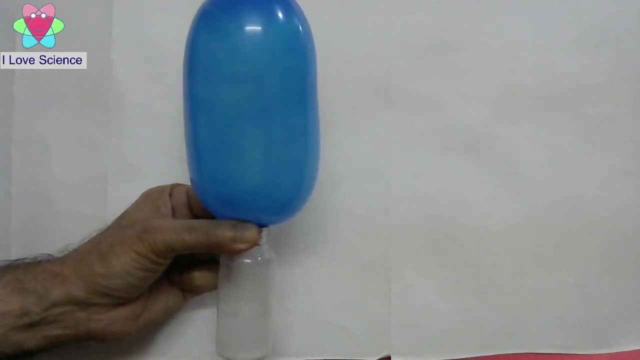 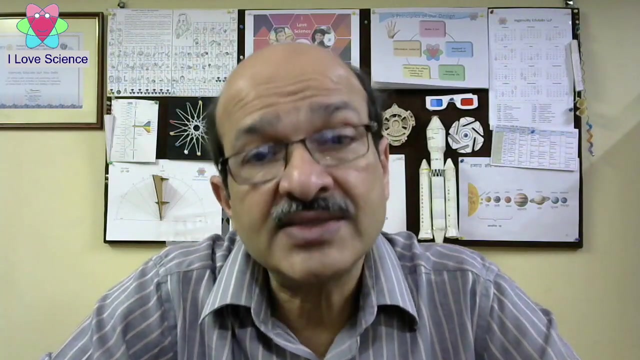 after 5 minutes. after 5 minutes, very active reaction of acid, citric acid and the base baking soda, and from that reaction so much of carbon dioxide gas got generated that it actually inflated the balloon so much. our next chemistry experiment is making some lava bottles. now, lava bottles may sound very dangerous. 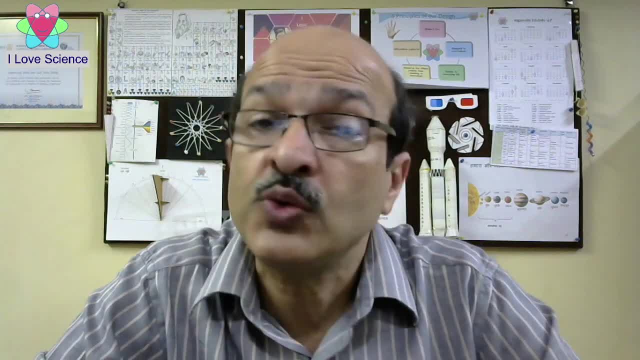 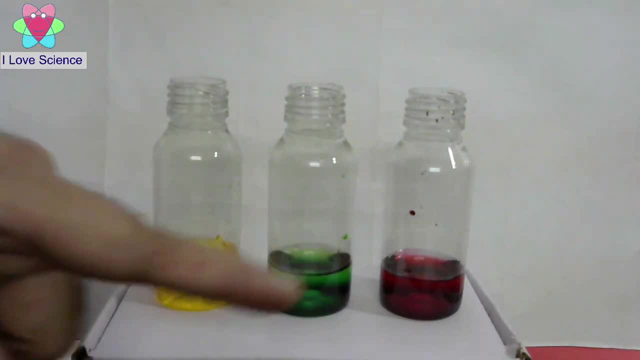 but they are very interesting and fun experiments and you can do these at home. so here in these small plastic bottles, we have taken some water and put food coloring in- that, okay, you can use any color, like ink or something. and then on top of this water we are adding some oil. i am using baby. 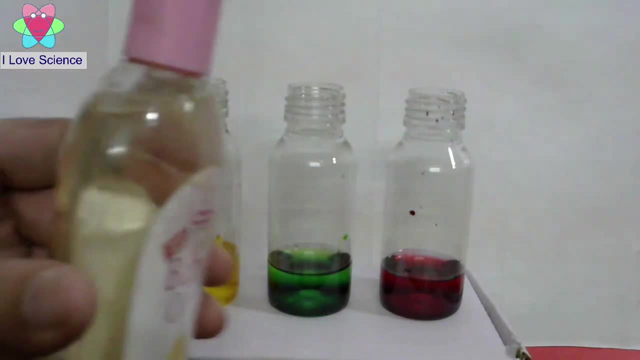 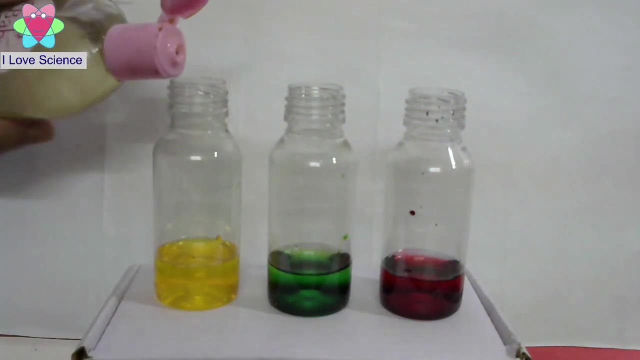 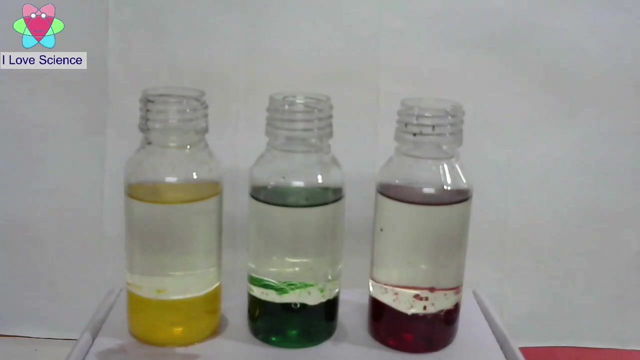 oil because it is transparent. it is not. it does not have any color. but you can use any other vegetable oil. but you should not use very dark color or yellow color vegetable oil so that the effect is nice. now you can see in three bottles we have colored water at the bottom and some transparent oil at. 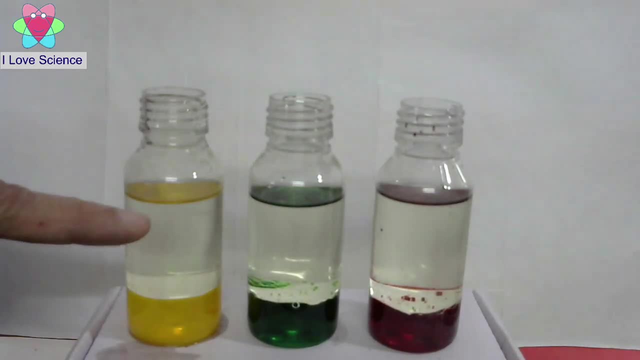 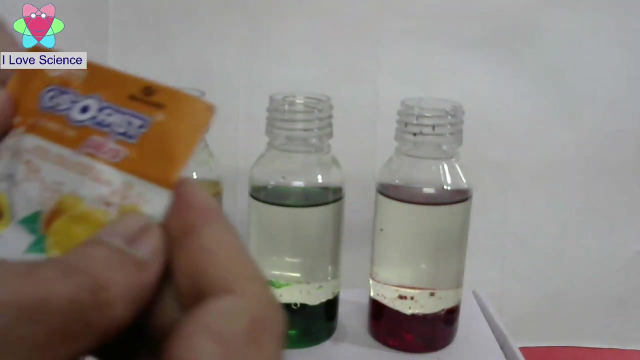 the top and you know that density of oil is lesser than water, so oil is floating on top of the water. now to do our chemical reaction, we are using some tablets which are which have same chemicals. like you know, they are available in different brand names and, basically, 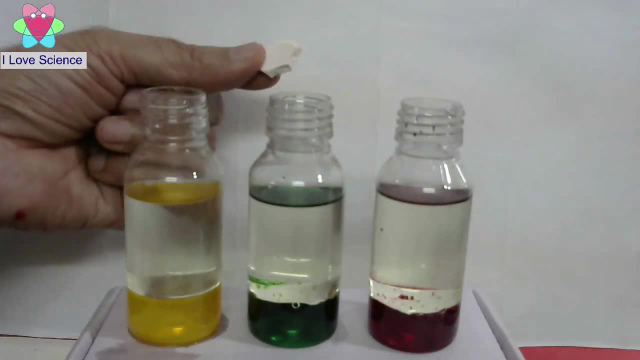 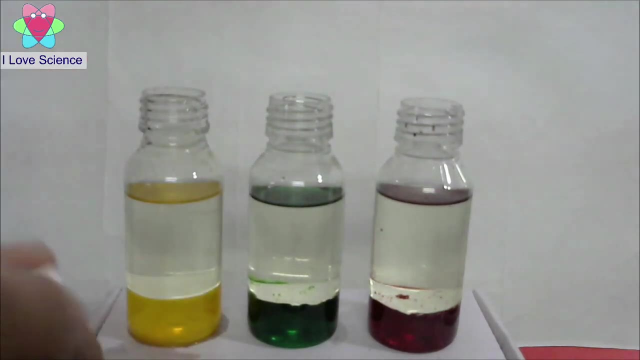 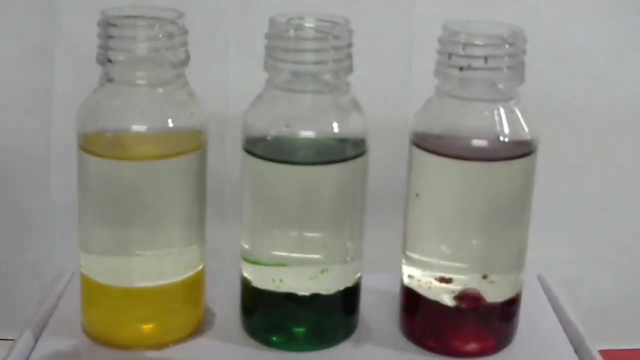 they have the combination of citric acid and baking soda. so when they go in the water they do the chemical reaction and then the carbon dioxide gas comes out. So now we will put small pieces of this tablet in each bottle and then see how does it work. 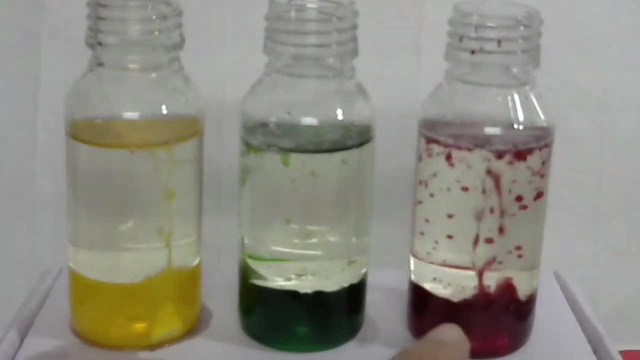 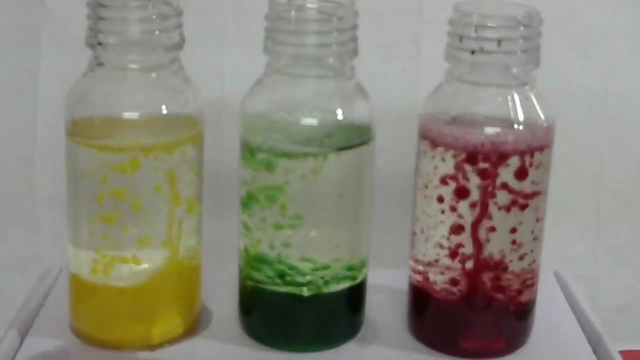 So you can see. when the tablet goes inside the bottle, the gas starts coming out and with the gas bubbles it brings some colored water along with them and those colored bubbles look like lava flowing inside the bottle. looks very beautiful. The reaction will keep happening as long as the citric acid and baking soda inside the 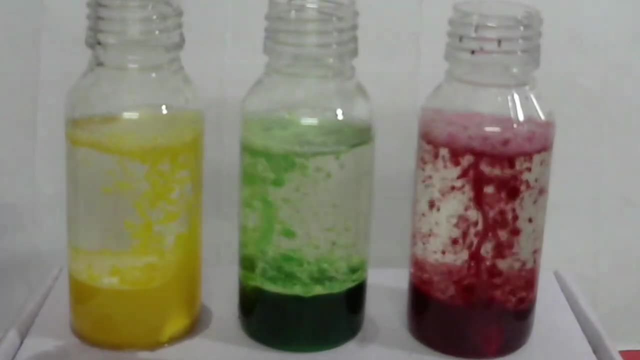 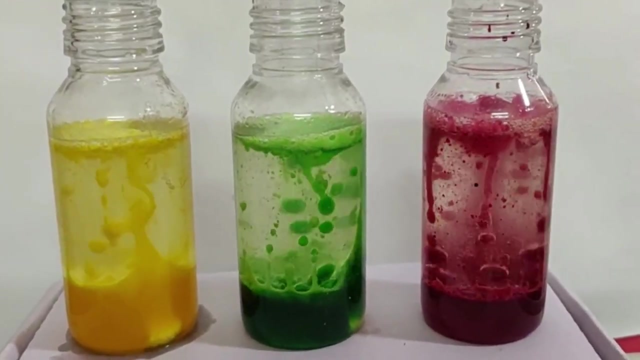 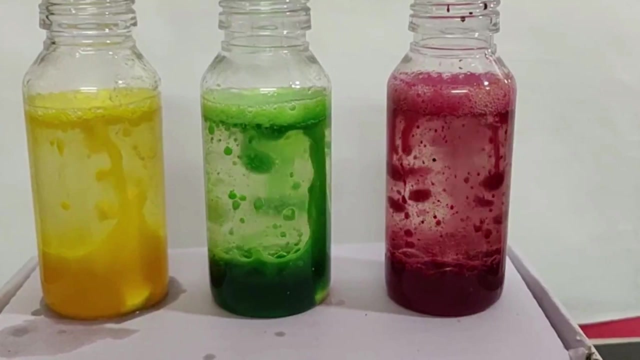 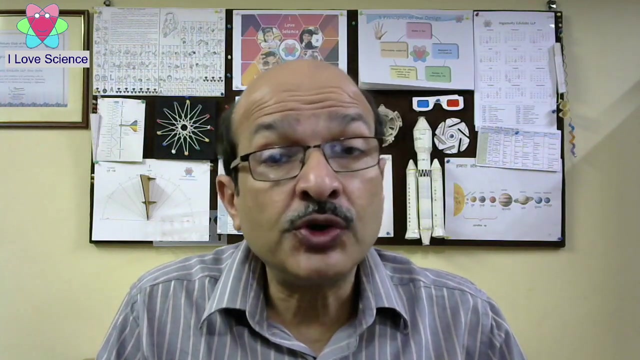 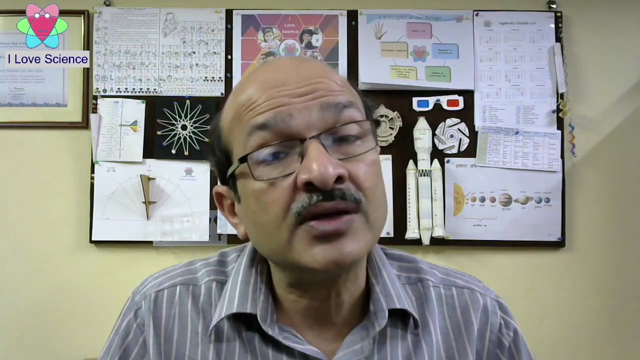 bottle are reacting. When the chemical reaction finishes, then these bubbles will stop and you can add another piece. For our next experiment, we will show you how to make a little volcano. This is a very popular experiment and lot of students do it as part of their school. 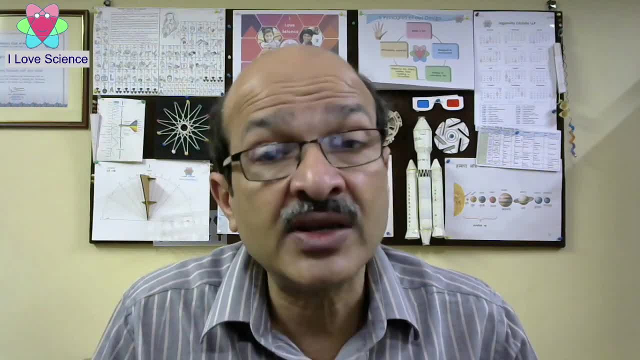 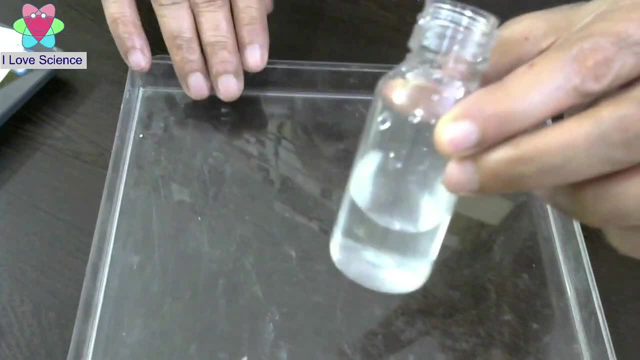 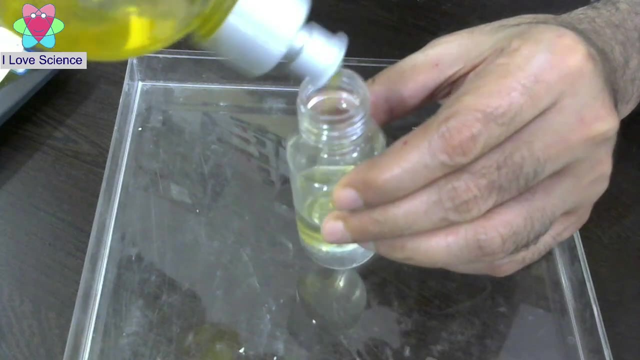 science. So let's see how can we do that in a very simple manner. So in this bottle we are adding some citric acid, So we have our citric acid solution ready. In this we will add a little bit of soap solution, so when bubbles come out they do not burst. 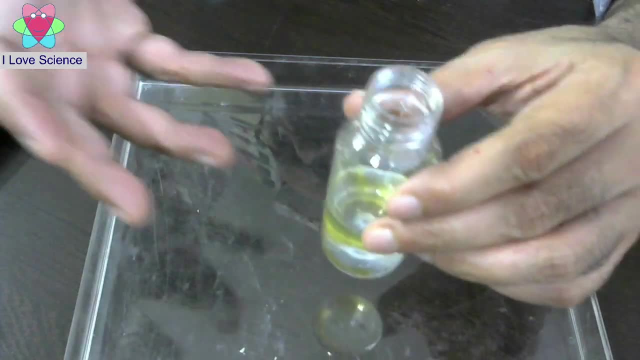 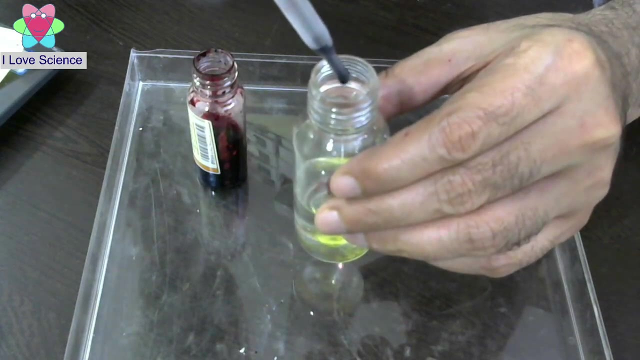 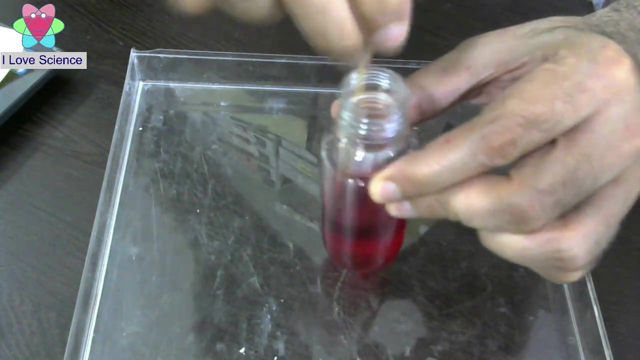 and they keep flowing in form of lava. We will also add some red food coloring into this. Just watch. One or two drops of that should be enough. Just mix this solution so that the liquid soap is mixed in the solution properly. So now just to repeat: what do we have in this bottle? 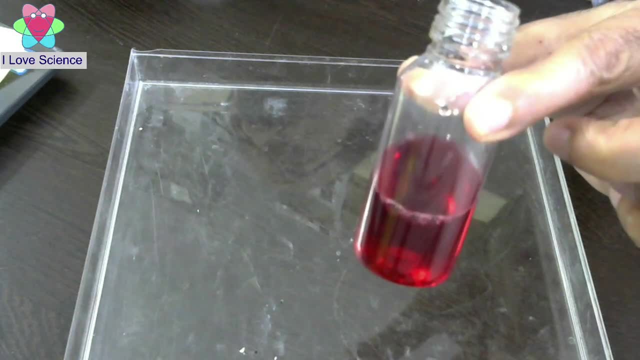 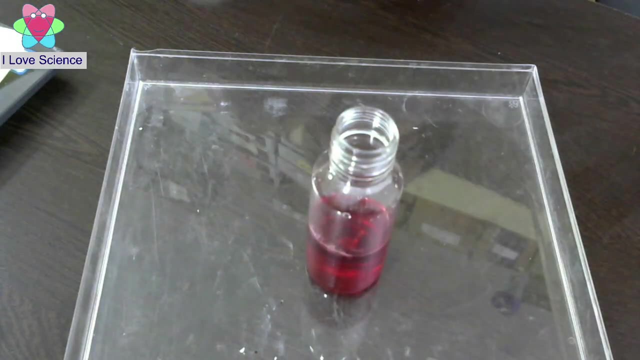 We have citric acid solution in water and we have added some red food coloring and a little bit of liquid soap. Now, when we add some baking soda into this, let's see what happens. So we will take some baking soda and add into the solution. 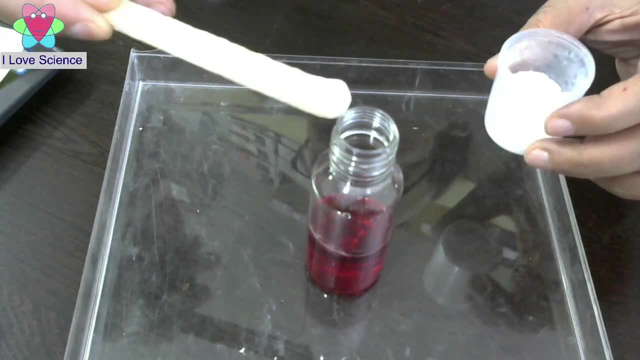 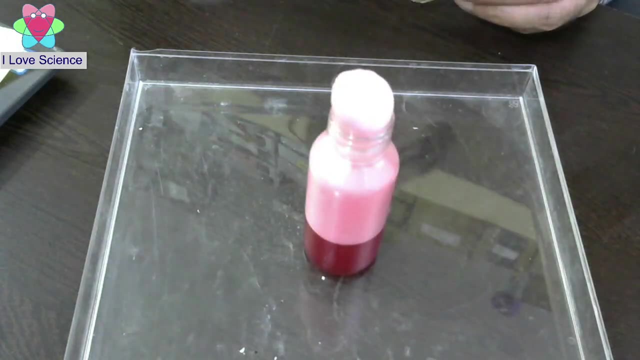 The gas should come out, But because we have soap solution, let's see what happens And then you will see the lava will start flowing, as if it's a volcano from which the volcano is erupting and the lava is flowing out of the bottle. 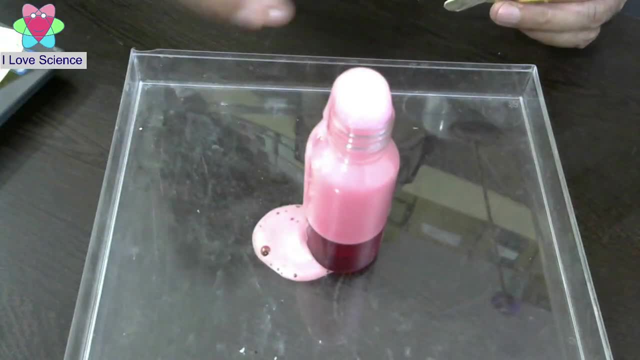 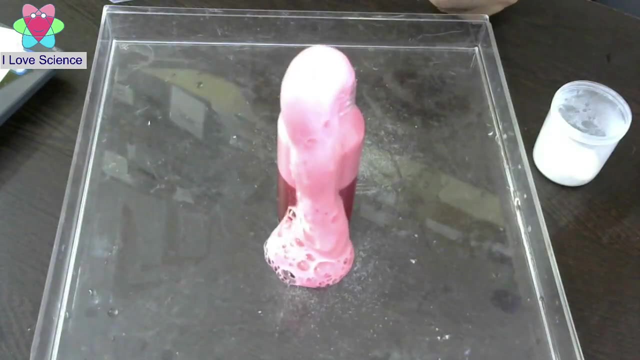 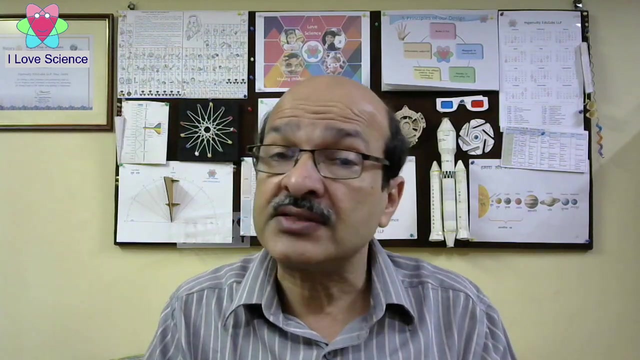 Now if you can make a little hill around that, so then it would look that the lava is coming out from the volcano which is on top of the hill. Our next experiment is called Elephant's Toothpaste, and this time we will not be using acid based reaction.